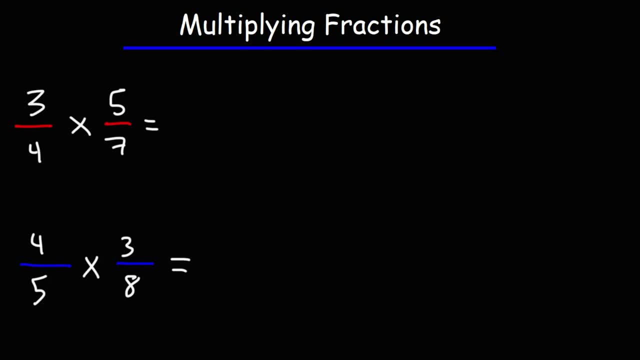 In this video, we're going to talk about how to multiply fractions. What you need to do is you need to multiply across. So you got to multiply the numerators together and the denominators together. Let's begin: 3 times 5 is equal to 15.. 4 times 7 is equal to 28.. So that's how you. 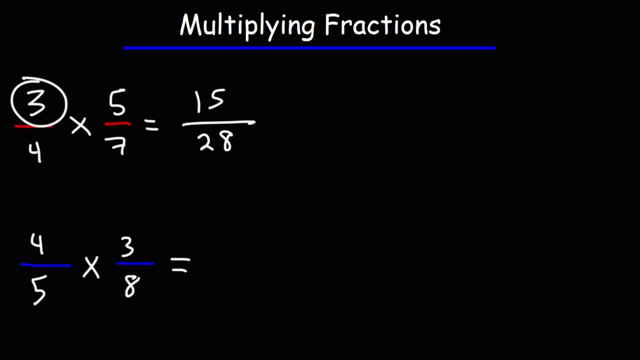 can multiply fractions. You simply multiply across. Now we can't simplify 15 or 28.. So this is as far as we can go for this problem. We can't reduce this fraction. Now what about the next one? What is 4 over 5 times 3 over 8?? To multiply these two fractions, we're going to do the same thing. 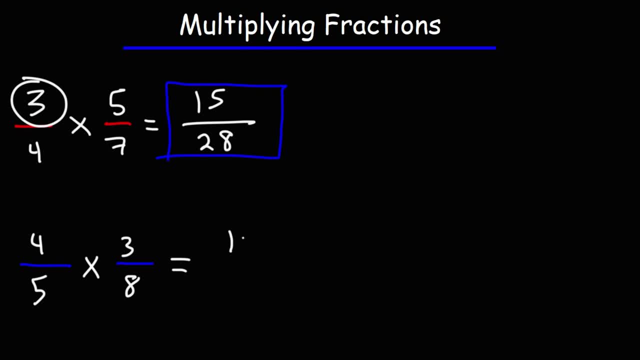 We're going to multiply the numerators 4 times 3 is 12. and then we're going to multiply the values in the bottom: 5 times 8 is 40. So our answer is 12 over 40. But we can reduce. 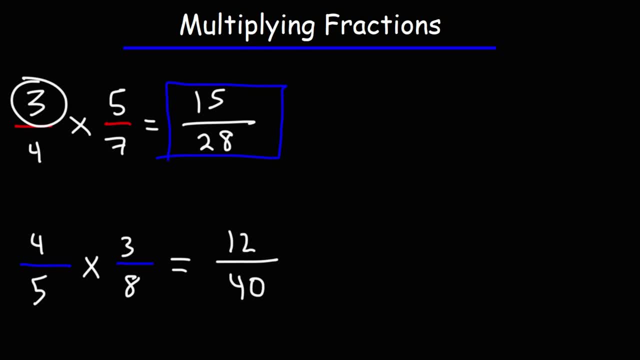 this fraction. Notice that both the 12 and the 40 are even numbers. So what we can do is we can divide both numbers by 2.. Half of 12 is 6.. Half of 40 is 20.. Now we can also reduce this fraction further, So we can divide both numbers by 2 again. 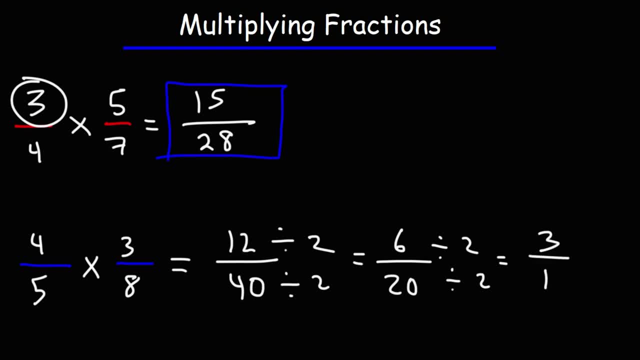 6 divided by 2 is 3.. 20 divided by 2 is 10.. So the final answer is 3 over 10.. By the way, for those of you who would like to reduce fractions faster, here's what you can do. 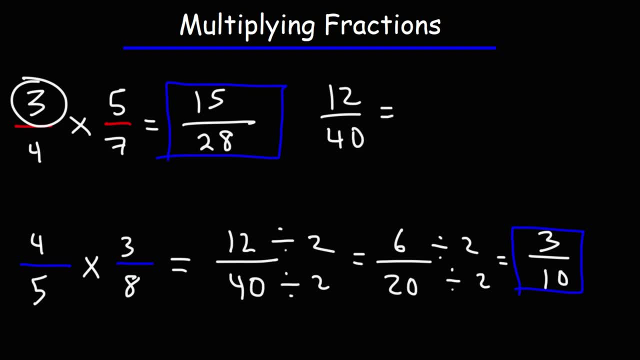 Going back to 12 over 40,. we could break down 12 into 4 and 3.. 4 times 3 is 12. 40. we can rewrite that as 4 times 10.. And notice that we can cancel a 4.. Doing it this way will. 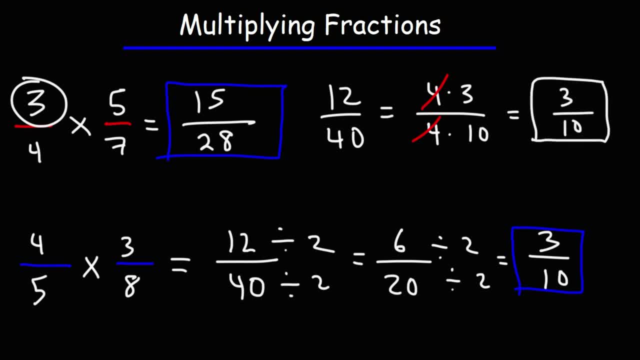 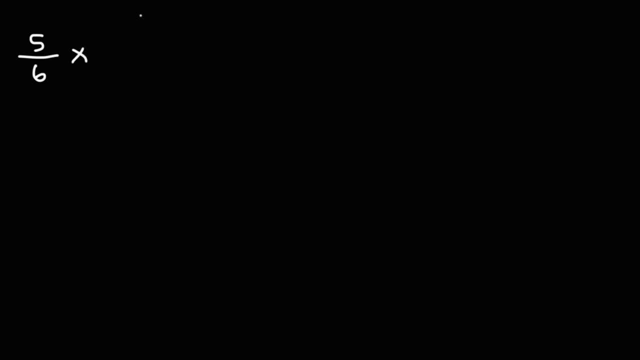 give us the same answer. The only difference is it's a lot faster. Now let's try some more examples. Let's say we have 5 over 6 times 4 over 9. Feel free to try that problem while I write down some more. 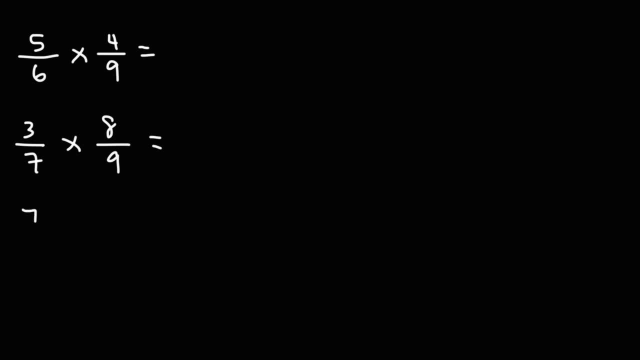 So go ahead and work on these four example problems. Starting with the first one, let's multiply 5 by 4.. 5 times 4 is 20.. And then we have 6 times 9, which is 54.. 20 and 54 are even numbers. We can reduce them. 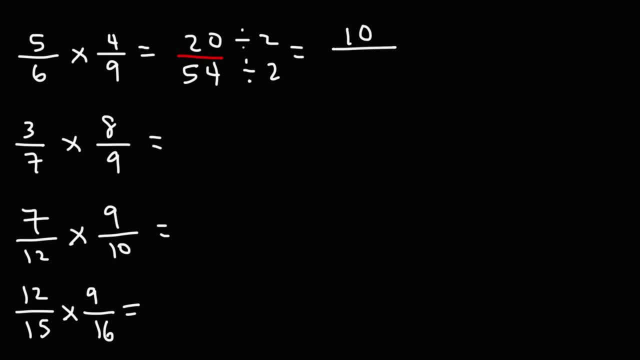 If we divide 20 by 2,, it will give us 10.. If we divide 54 by 2,, it will give us 27.. So the answer is 10 over 27.. Now let's try the next one. 8 times 8 is 24.. 7 times 9 is 63.. 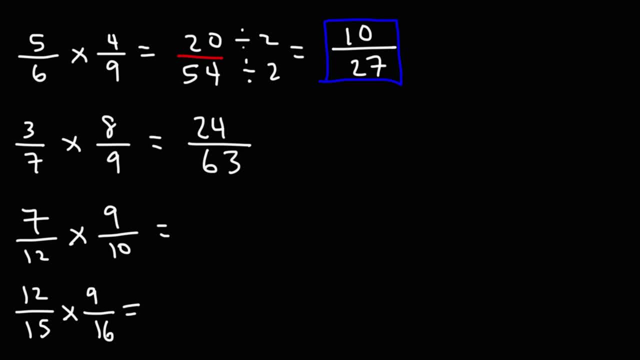 Now, we can't divide 63 by 2, but 24 and 63, they're divisible by 3.. 24 divided by 3 is 8.. 63 divided by 3 is 21.. And that's as far as we can go for this problem. 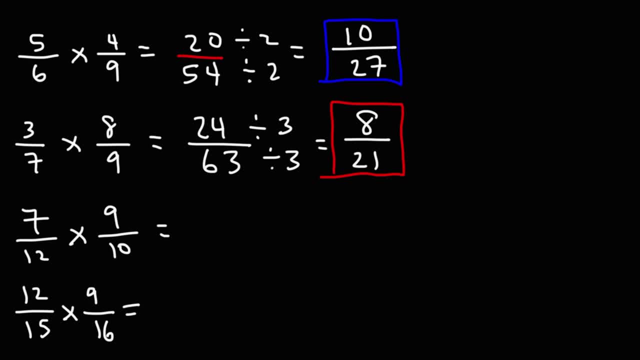 So the answer is 8 over 28.. Now let's try the next one. 7 times 9 is 63.. 12 times 10 is 120.. We could divide both of these numbers by 3.. We know that 63 divided by 3 is 21.. 120 divided by 3 is 40. 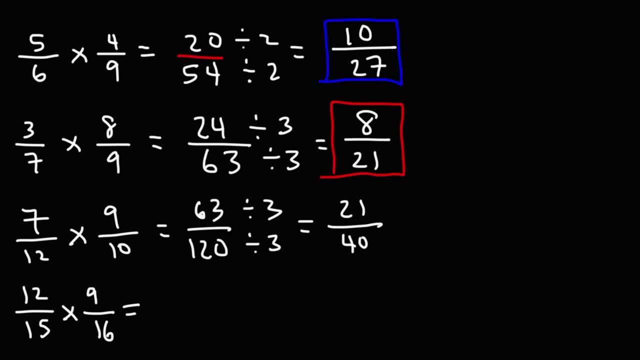 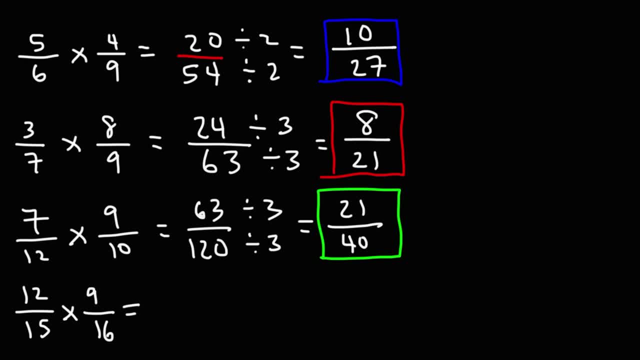 And that is about all we can do for this problem. So it's 21 over 40.. Now for the next one, what you can do to make it easier, because if you multiply 12 by 9, you're going to get a big number, and then you have to reduce it. 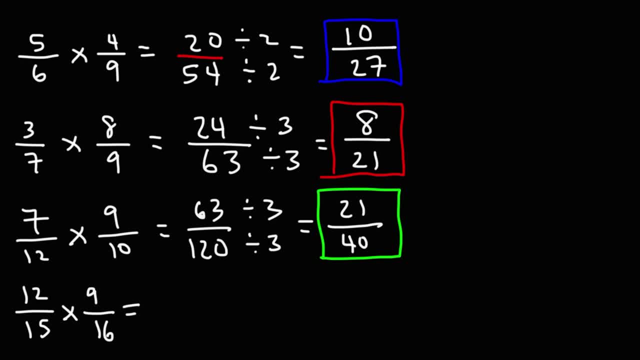 Now for the next one: what you can do to make it easier, because if you multiply 12 by 9, you're going to get a big number, and then you have to reduce it. Instead, I'm going to show you another way in which you can get the same answer, a much simpler way.